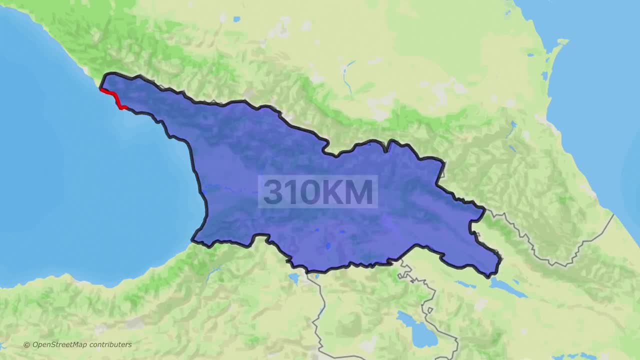 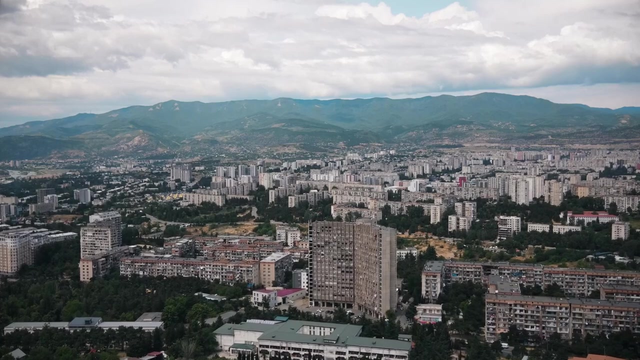 is 69,700 square kilometers and its coastline is 310 kilometers and has a population of about 3,700,000 people, which is ranked 132.. Considering that Georgia has many natural resources, including oil and gas, the loans to the climate of this country is suitable for the growth of products. 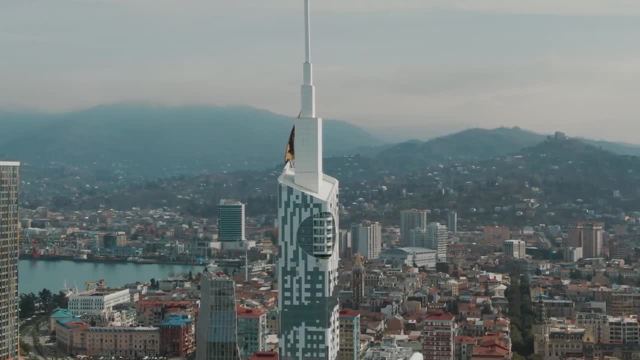 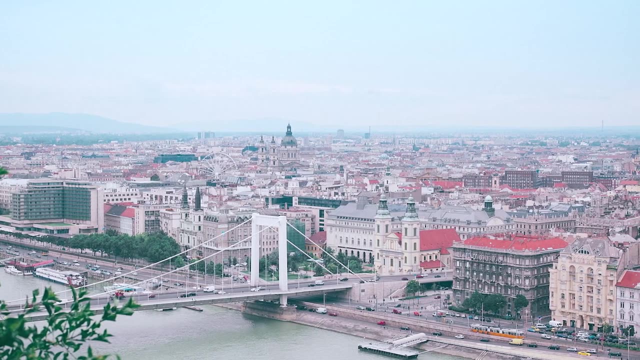 such as wine grapes and tea leaves, which are some of their most valuable exports. But despite all this potential wealth, Georgia is not considered one of the richest countries in the world. In fact, it is not even among the top 50 richest countries on earth, which has various reasons why Georgia is. 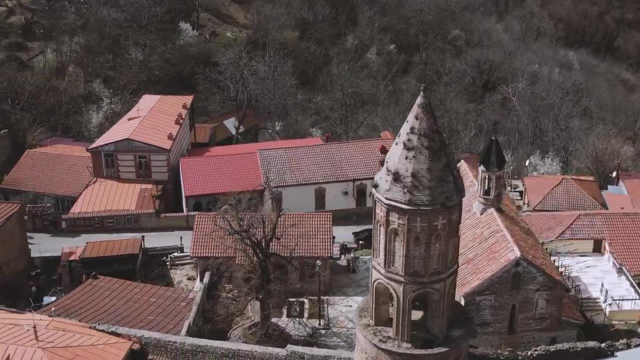 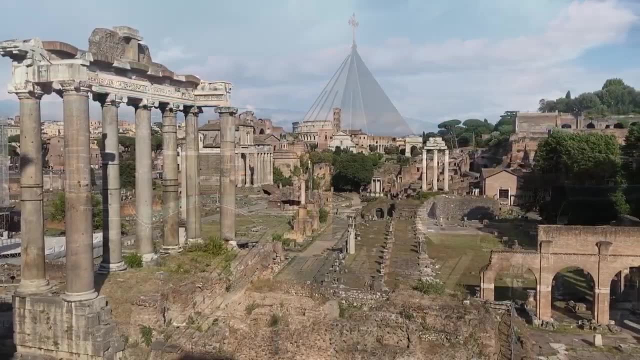 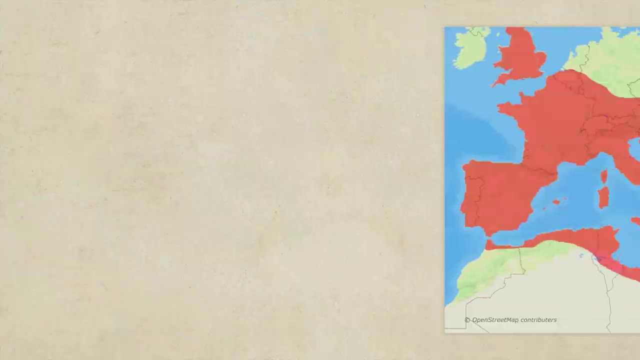 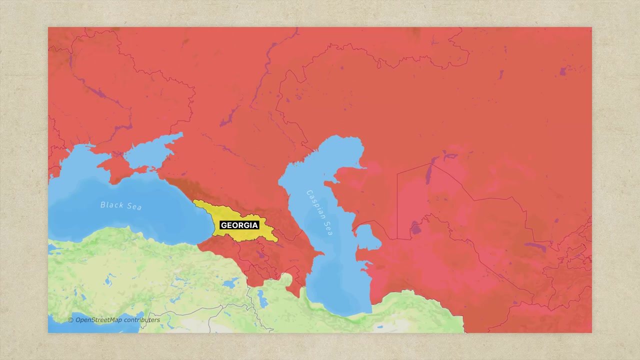 not a rich country. So let's get started. The history of Georgia is a long and complicated one. The country has been occupied by different empires and kingdoms, including the Roman Empire and various Iranian dynasties, And also in the 19th century, Georgia joined Russia and became part of the Russian Empire, And after 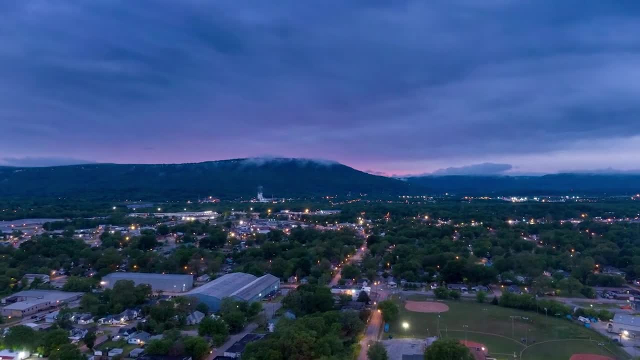 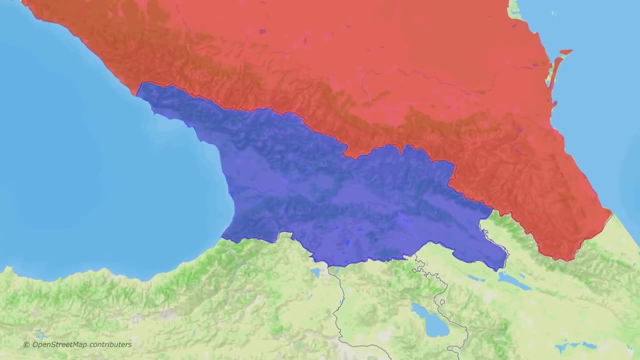 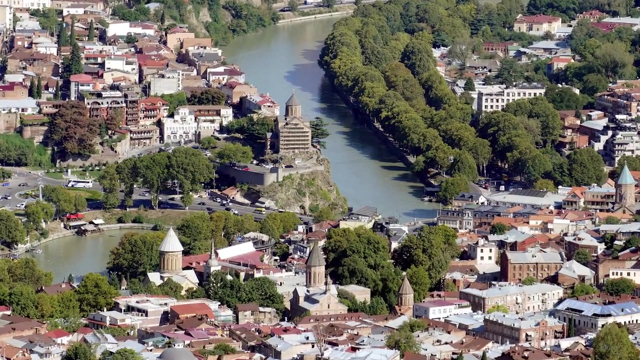 the Russian Revolution in 1917, Georgia declared its independence and established a democratic republic. However, this independence was short-lived, as Georgia was invaded by Soviet Russia in 1921 and joined the Soviet Union. During the Soviet rule, Georgia faced political repression. economic problems and cultural assimilation. In 1991, after the collapse of the Soviet Union, Georgia regained its independence and adopted a new constitution. However, due to weak infrastructure and political instability, it also faced new challenges, such as ethnic conflicts. 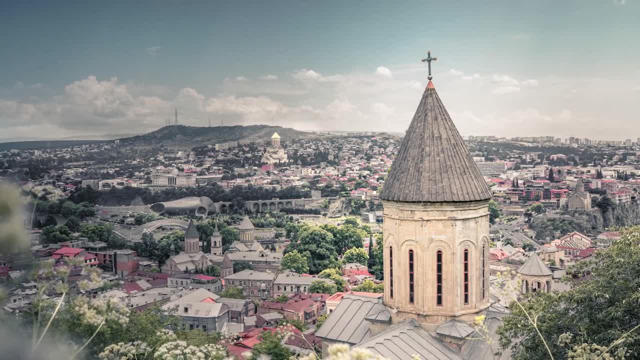 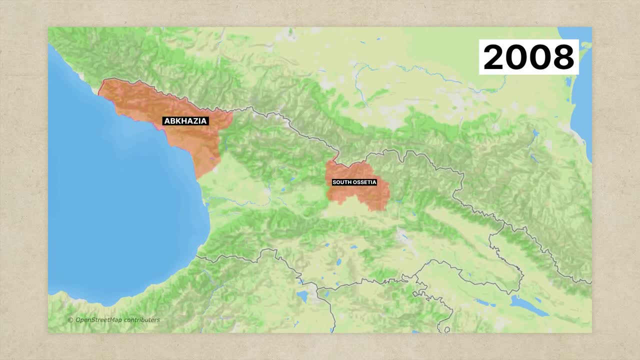 civil wars and civil wars. However, due to weak infrastructure and political instability, it also faced new challenges, such as ethnic conflicts, civil wars, separatist movements and economic crises. 2008 was also due to a long-running dispute over the two breakaway regions of Abkhazia and South Ossetia in Georgia, which triggered Russian 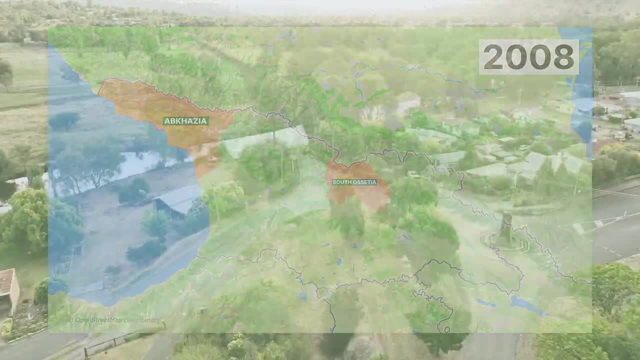 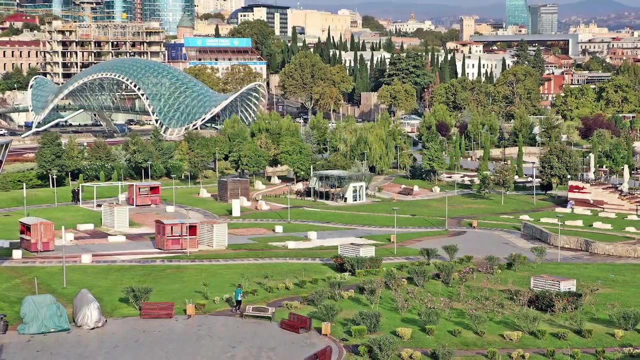 economic embargo and weakened the country's economy. In fact, these regions were supported by Russia in the early 1990s. Russia had declared independence from Georgia, but Georgia considered them part of its independent territory and tried to regain control of them. As a result, 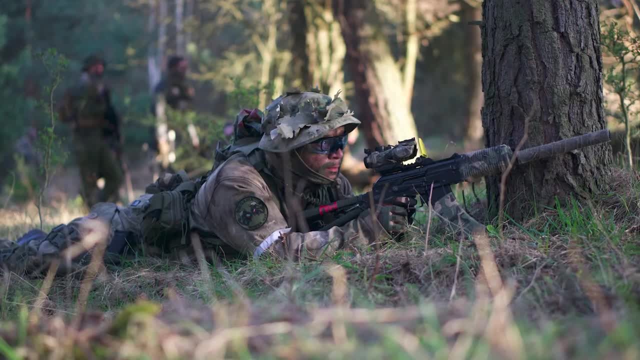 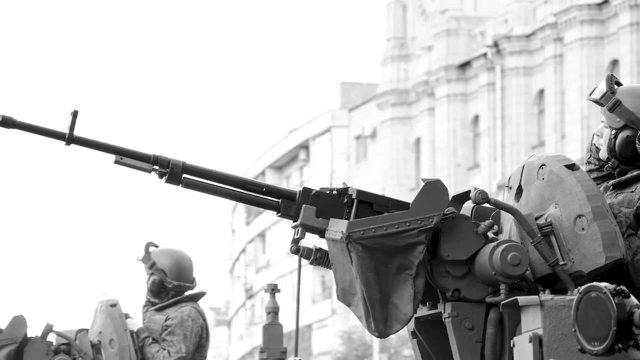 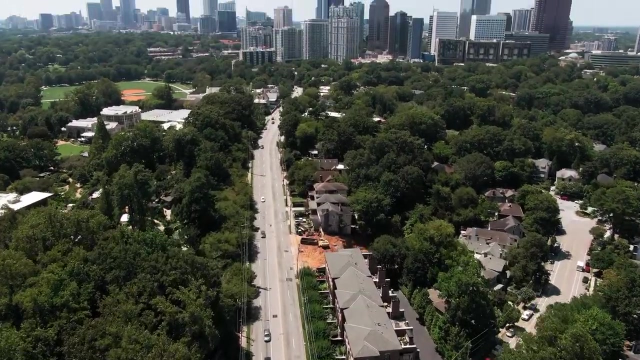 in August 2008,. after months of escalation of tensions and clashes, Georgia started a military operation to recapture South Ossetia, and Russia responded by sending troops and tanks to South Ossetia and Abkhazia, as well as bombing Georgian cities and infrastructure. The war lasted for five. 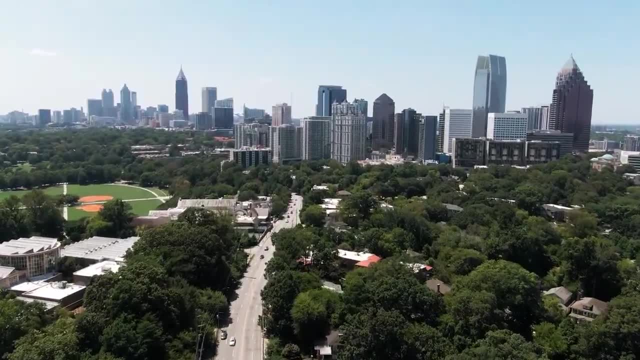 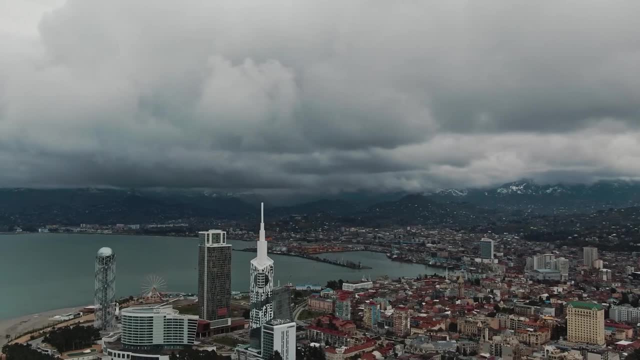 days and ended with an armistice agreement procured by France. One of the gods and goddesses of the war was that Russia recognized Abkhazia and South Ossetia as independent states, while most of the community continued to support the territorial integrity of Georgia. Therefore, Russia imposed: 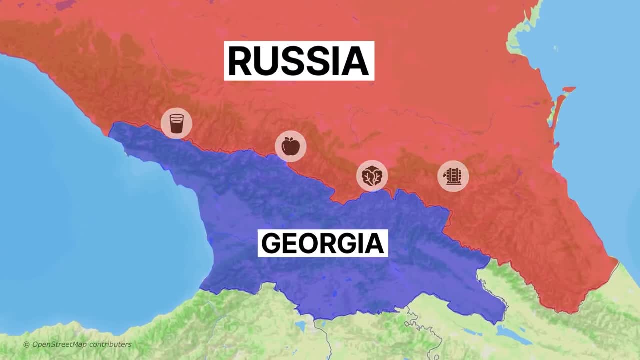 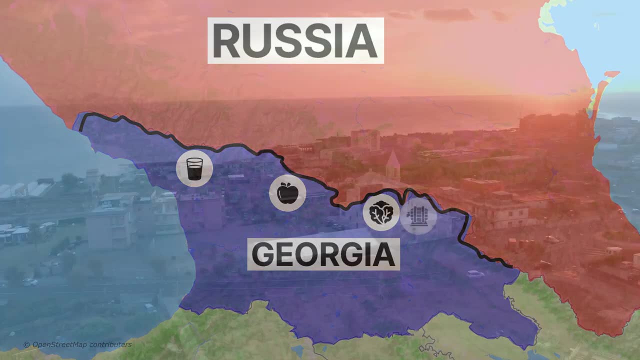 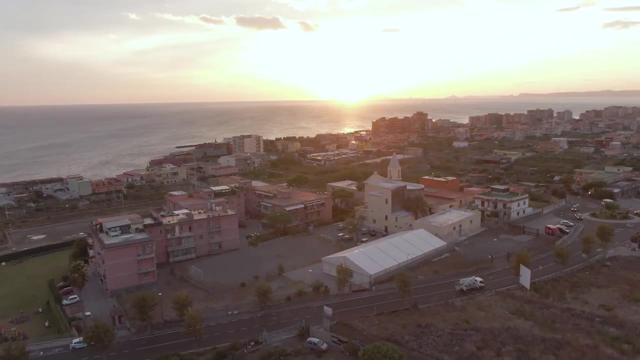 an economic embargo on Georgia and cut off its trade relations and banned Georgian products such as wine, mineral water, fruits and vegetables from entering the country's markets. This economic embargo has a significant impact on the Georgian economy, Already suffering from war-related damage. Georgia lost about $1 billion in trade revenue due to the Russian ban. According to some estimates, the sanctions also cost thousands of Georgian workers who exported remit from Russia. Of course, Georgia's right to cope with the economic crisis by diversifying its business. partners and attracting foreign investment, and also received significant financial aid from Western countries such as the United States and the European Union. But despite these efforts, the growth of Georgia's GDP decreased from 9% in 2007 to 3.8% in 2009.. The economic embargo lasted. 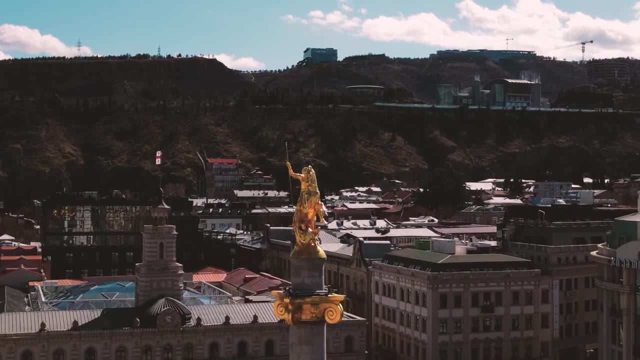 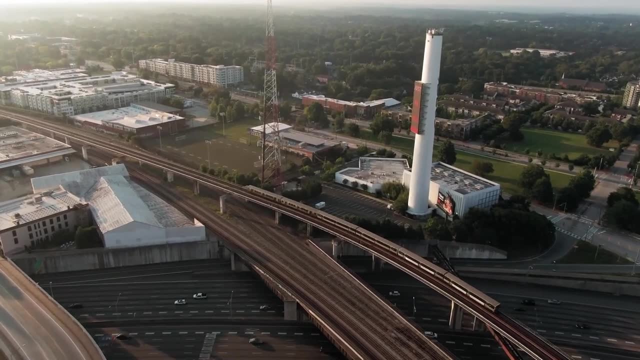 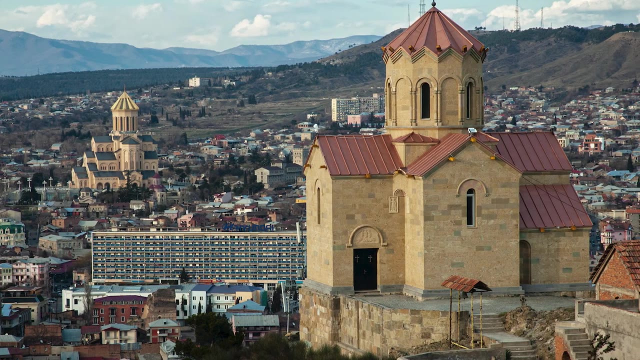 Russia lifted some of its restrictions and Georgian products after both countries joined the World Trade Organization, but political relations between Russia and Georgia have remained stable to this day. It is tense, especially regarding the situation in Abkhazia and South Ossetia. Today, Georgia has formed a parliamentary republic with a multi-party system. 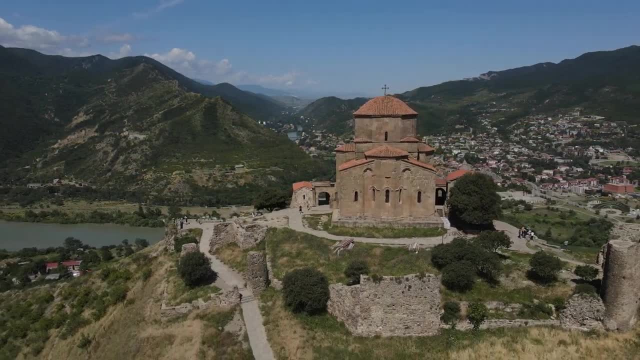 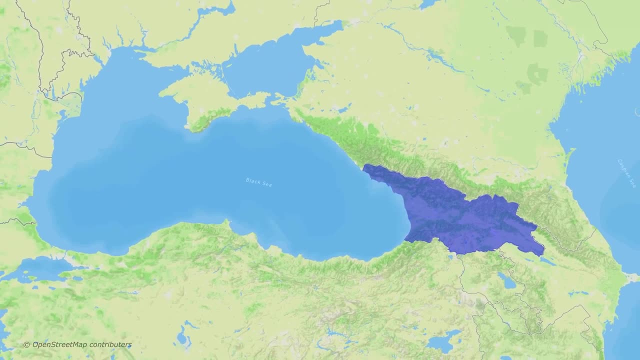 which must overcome many challenges to create a strong economy. This means that it cannot directly access the international markets by sea. If you look at the map, the only sea route of Georgia is the Black Sea, which is an enclosed sea and has no weighted ocean, and Georgia has 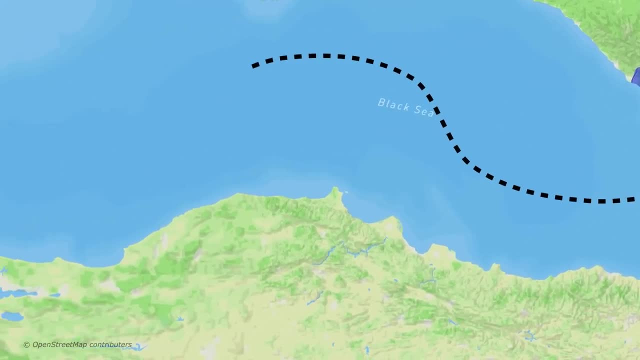 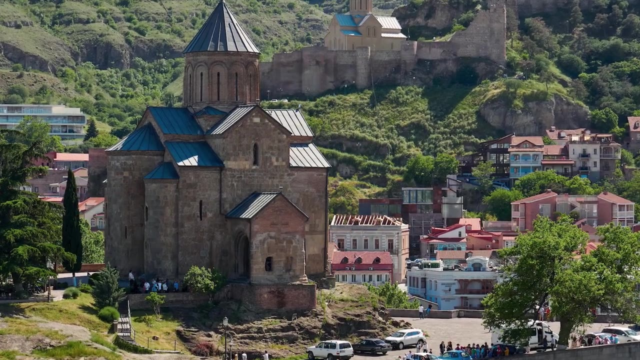 to reach the ocean through this sea, facing an obstacle like Istanbul, Turkey, which is the border between the Black Sea and the Mediterranean Sea. Therefore, in order for this country to have access to international markets, it must use the territory or waters of other countries. 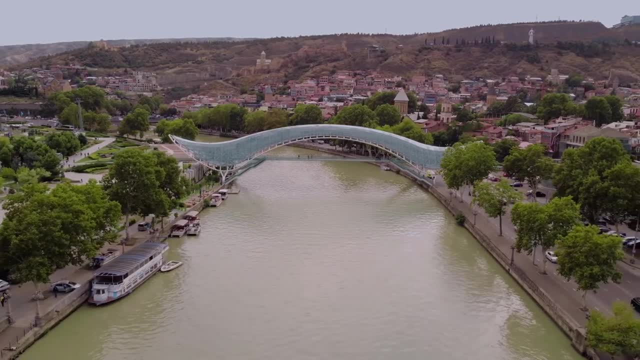 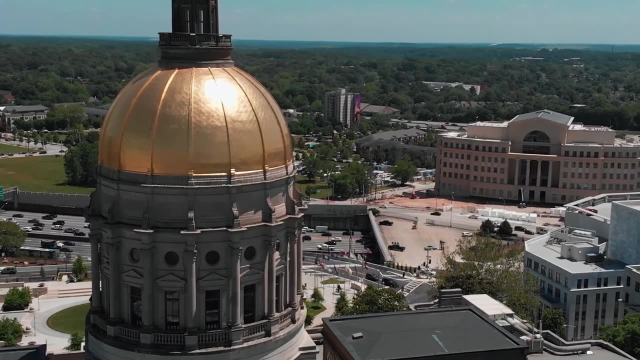 which makes the exchange of goods and services more expensive for Georgia than countries that have direct access to oceans or sea. Georgia also faces challenges that the United States and other European countries face. For example, the United States and other European countries face challenges that prevent potential investors from entering its market. 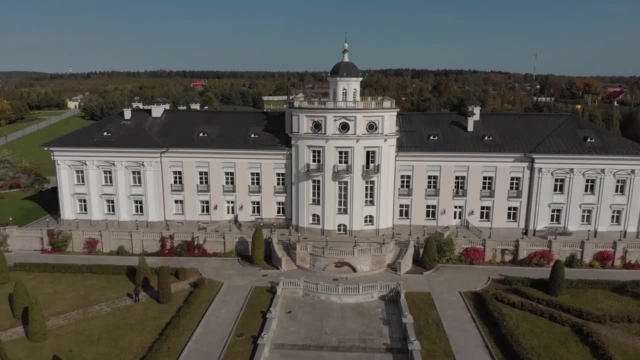 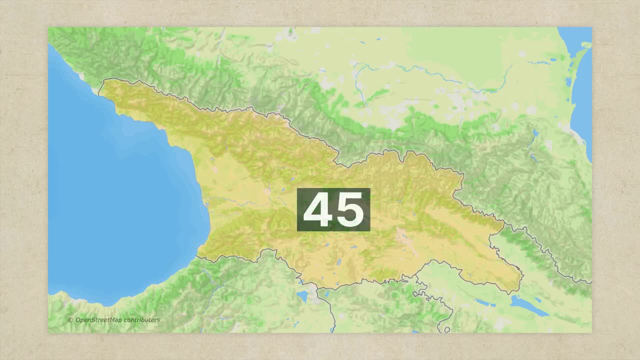 One of these challenges is corruption, which is still a serious problem in some sectors and institutions. Due to the international transparency of Georgia, its currency ranks 45 in the Corruption Perceptions Index, which measures the level of public sector corruption in a country. 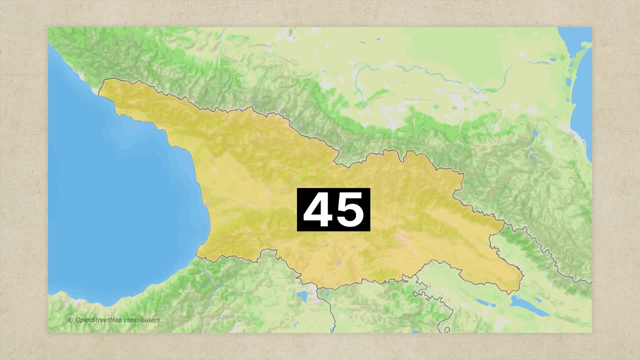 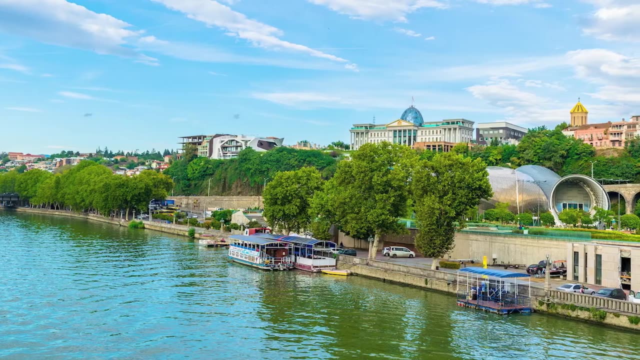 This is a relatively good score compared to other countries in the region, but it also shows that there is still room for improvement. Also, one of the main sources of corruption in Georgia is the use of offshore companies by some business allies and politicians. Offshore companies are entities registered in jurisdictions with. 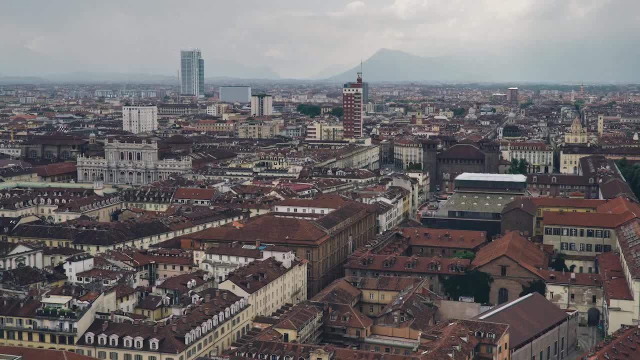 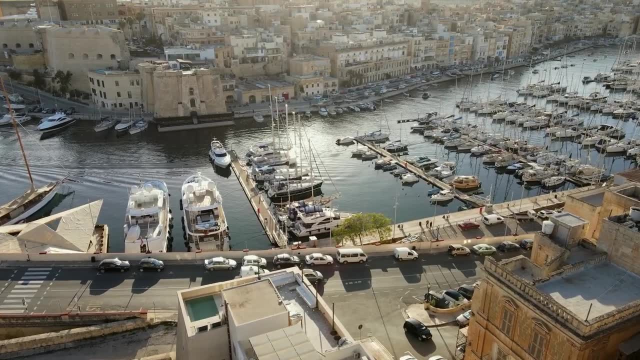 law or no taxes and WIC regulations, and they can be used for legal purposes, such as tax optimization or asset protection, but can also be used for illegal activities such as money laundering, tax evasion or hiding conflicts of interest, According to Transparency International Georgia. 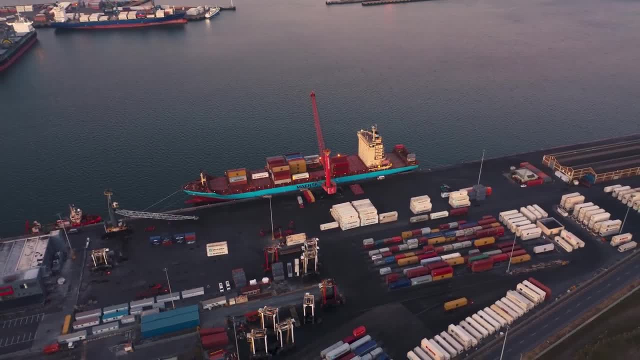 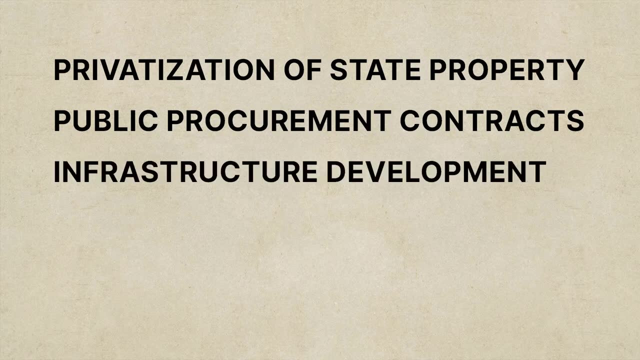 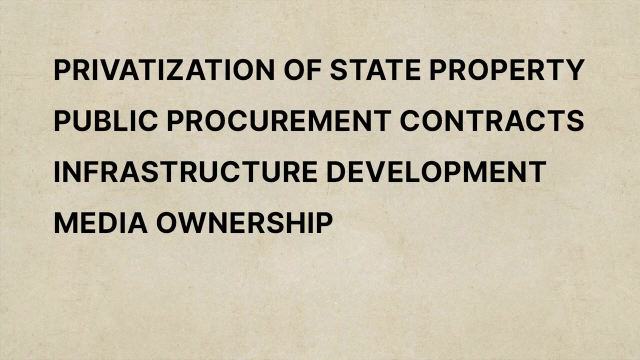 offshore companies are involved in many large transactions and projects in Georgia, such as the privatization of state property, public procurement contracts, infrastructure development or media ownership. yet the identity and ownership structure of these offshore companies are often obscure and difficult to track. This creates the risk of corruption because it allows 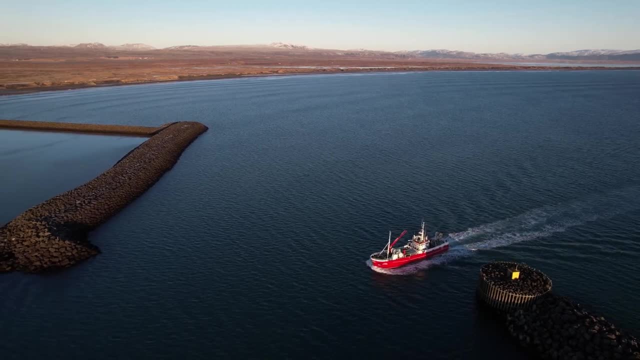 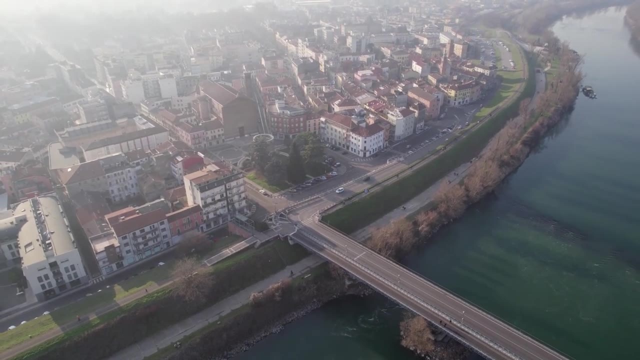 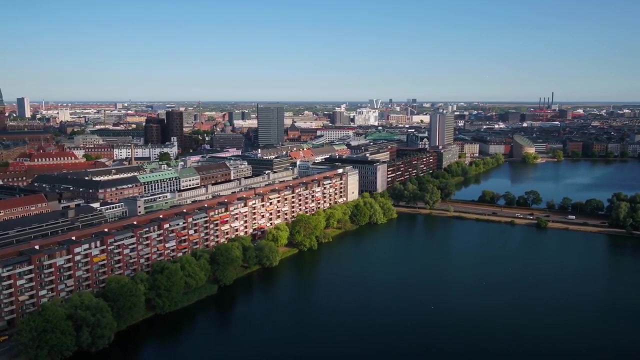 some individuals or groups to influence public decisions or policies without disclosing interests or paying taxes, and it also undermines public trust and accountability because it prevents for citizens to know who benefits from public resources. The use of offshore companies also discourages foreign investors from investing in Georgia. 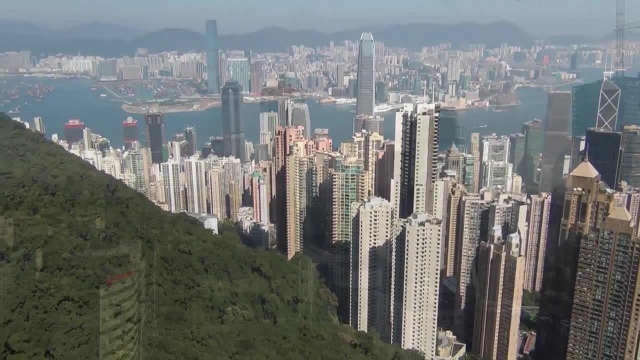 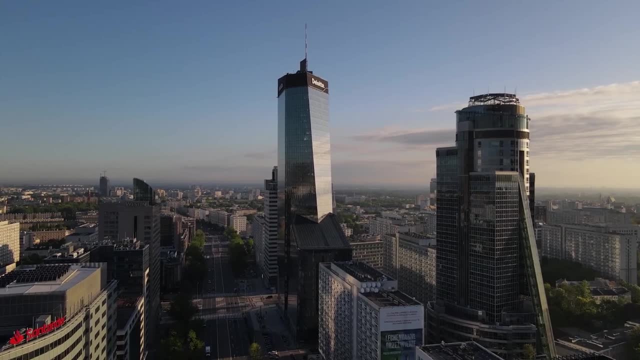 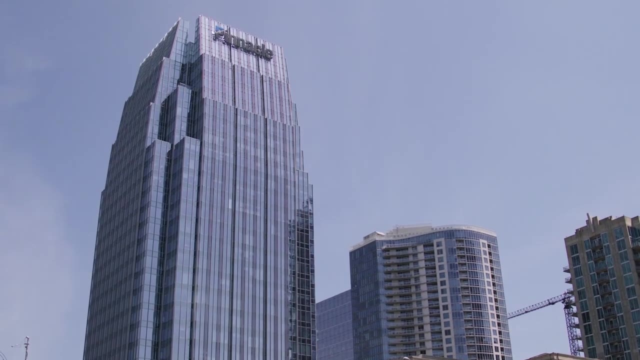 as it creates an uneven playing field and reduces transparency, and foreign investors may face unfair competition from local businesses that hire foreign companies use the country to avoid taxes or regulations. They may also face legal uncertainties or credit risks if they partner with entities linked to foreign companies. 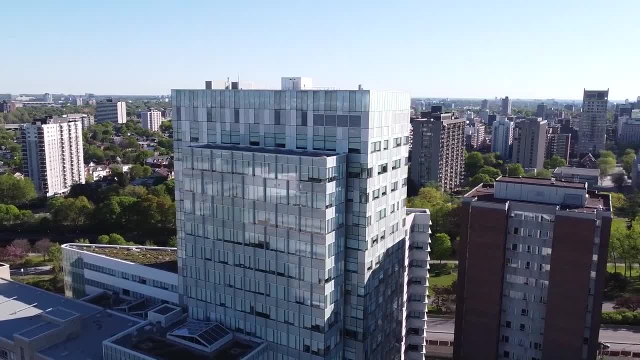 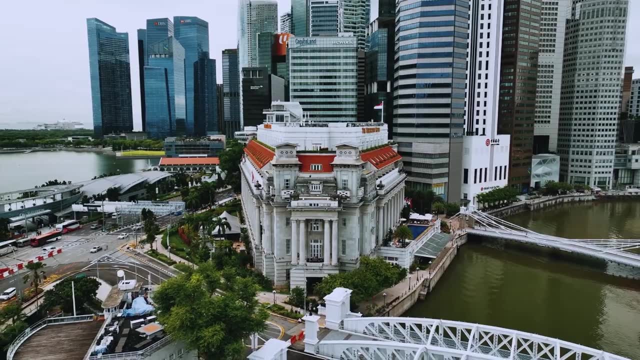 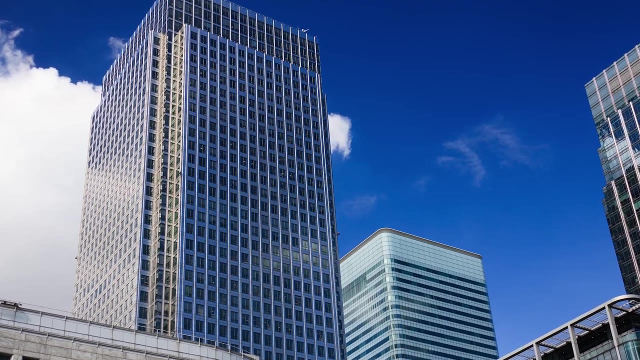 So if Georgia wants to attract more foreign direct investment and boost its economic growth, it needs to address the issue, address corruption related to offshore companies and Transparency International. Georgia recommends that the country should follow the recommendations of the Organization for Economic Cooperation and Development's 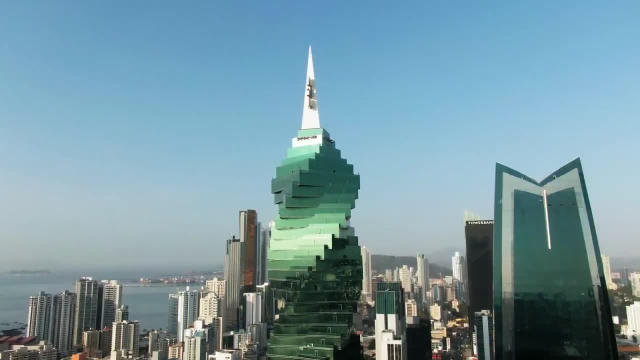 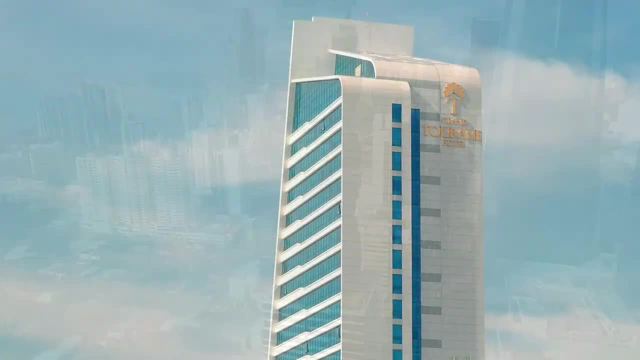 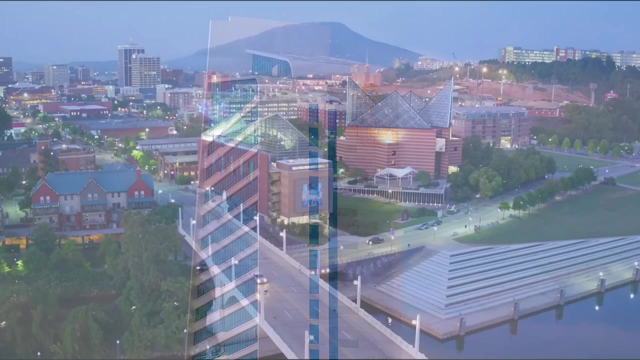 Anti-Corruption Network and disclose to beneficial owners of offshore companies in order to prevent these and cause let foreign companies invest in this country. Georgia's international relations also have a significant impact on the country's economy. One of the most important factors is trade agreements that allow countries. 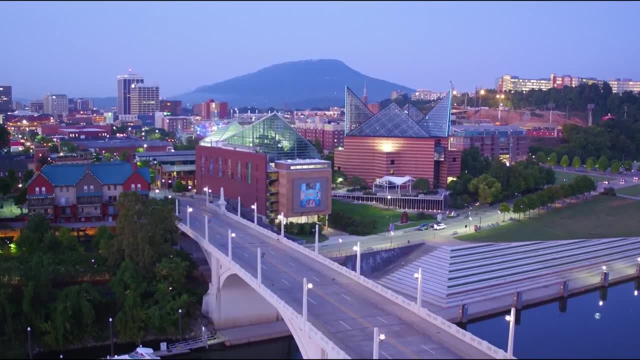 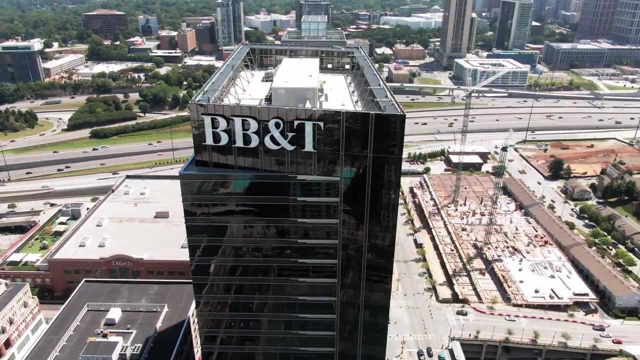 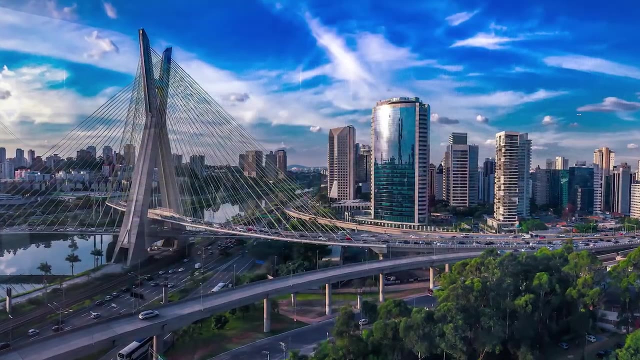 to exchange goods and services without tariffs or other restrictions. Georgia has several such agreements signed with other countries around the world, including Turkey and Azerbaijan, which arrangements have contributed to economic growth by allowing Georgian businesses access to markets they would otherwise have been unable to access. However, 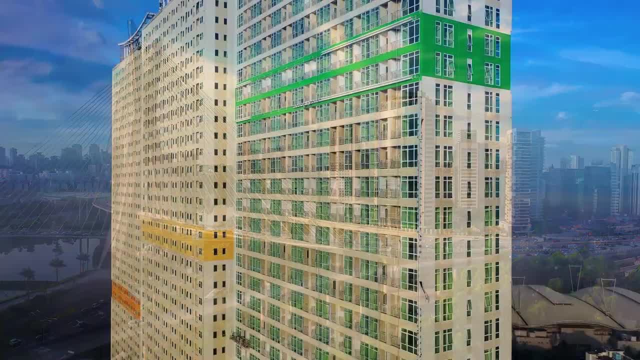 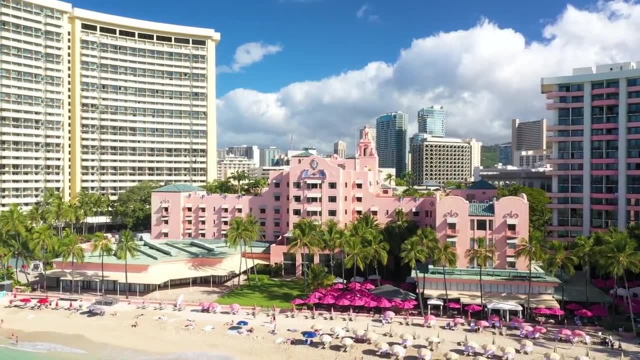 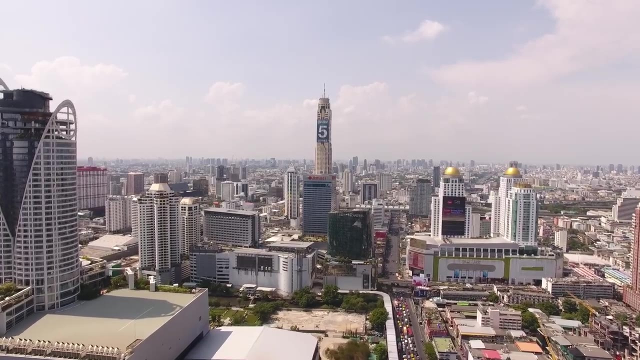 they have also made it difficult for some industries in Georgia because they come directly with foreign imports that face no barriers when entering domestic markets, and international aid programs can also affect the performance of an economy. In the end, the main point is that Georgia has a lot of potential to improve its economy and should be able to avoid the problems that. 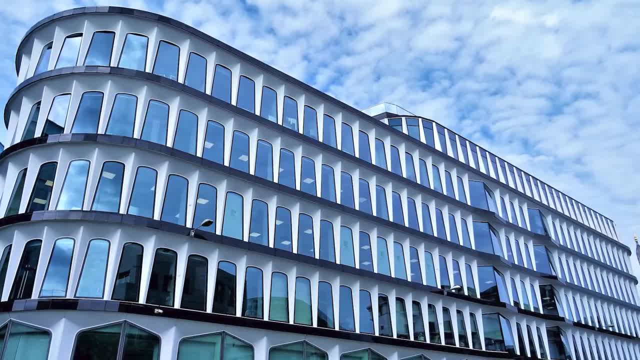 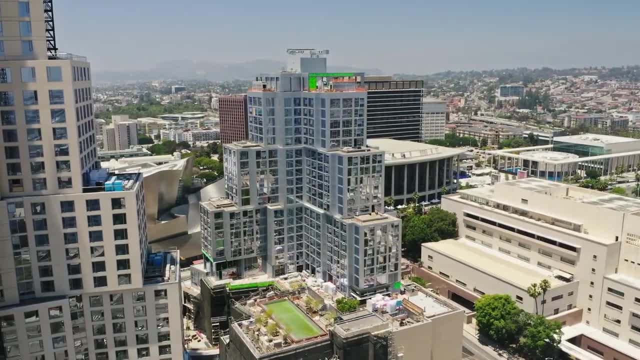 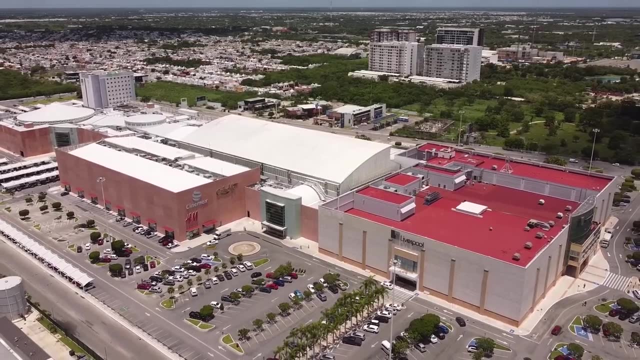 I mentioned in this video, in order to be able to flourish its economy. I recommend that you see me, because Luxembourg is the best country in terms of domestic crude production, which has been able to perform two times better than the United States. Finally, if you liked this video, please like it and watch the recommended video. 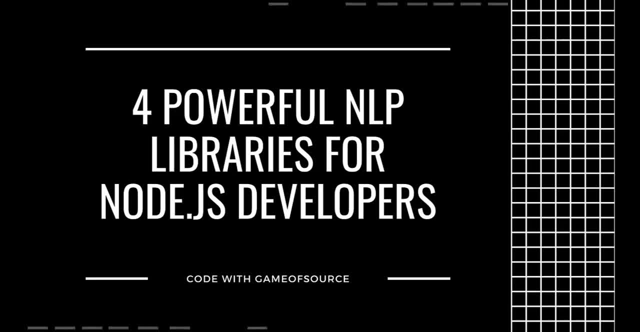 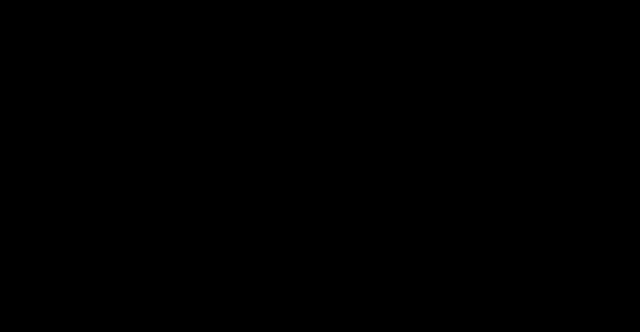 Hey and welcome to this video where we'll go through some of the most popular Nodejs NLP modules. Natural Language Processing libraries may help you analyze, comprehend and synthesize human language content in a developer-friendly manner. Let's get started by looking at four of the most popular Nodejs packages for NLP. 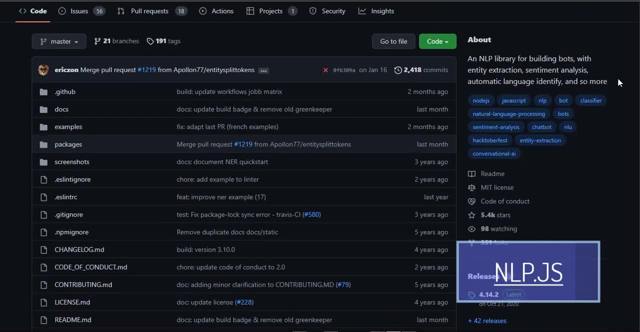 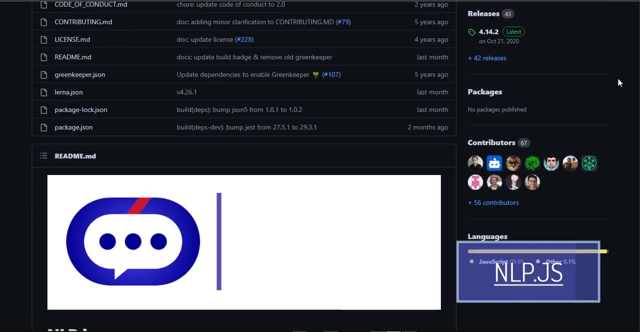 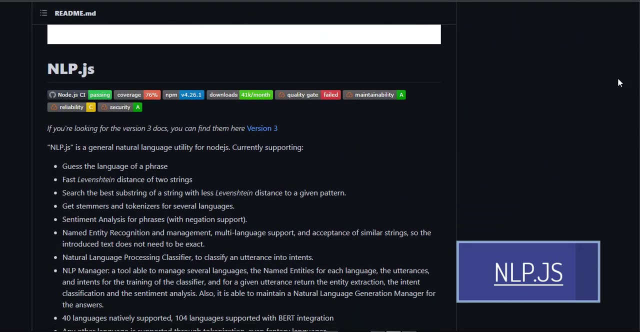 The first is NLPjs, which was created by the AXA group. Tokenization, sentiment analysis, entity identification and other functionalities are included in this library. NLPjs's ability to handle many languages is one of its distinguishing qualities, giving it a versatile solution for worldwide applications. 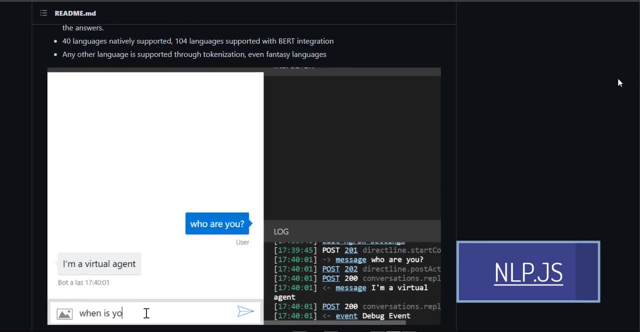 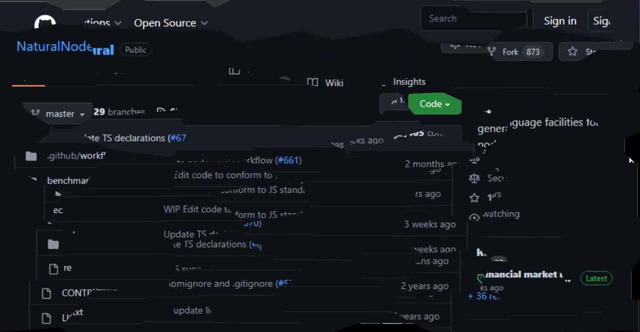 It also provides a user-friendly and well-documented API that is simple to use for both novices and specialists in NLP. Natural is the next-generation of Nodejs. Natural is the next-generation of Nodejs. Natural is the next-generation of Nodejs. 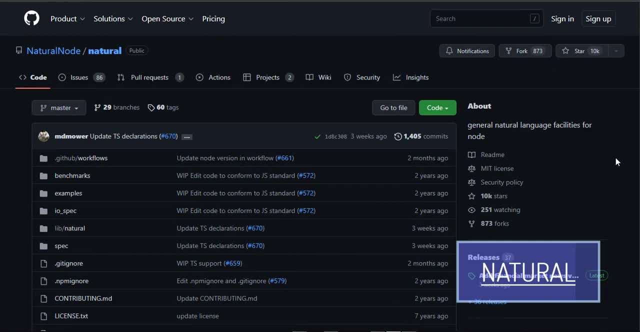 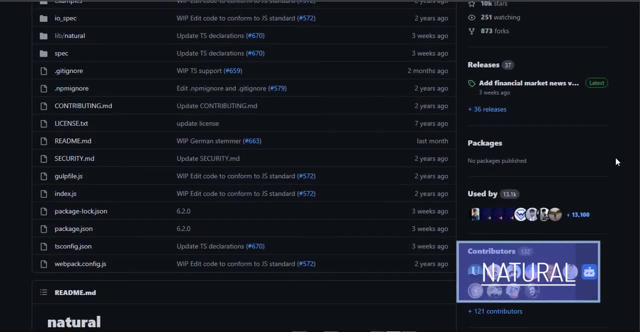 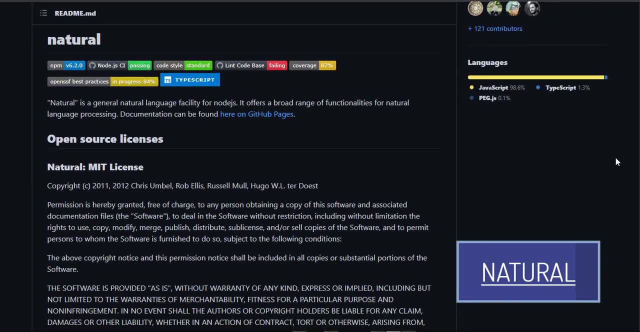 Natural is a popular Nodejs framework noted for its simplicity of use and versatility. Total pros are 음 basis and breadth and variety of abilities that areíll precladım for the usr% andresse тысяч个ne. Although different- kabnapWow, she's not so bad in.